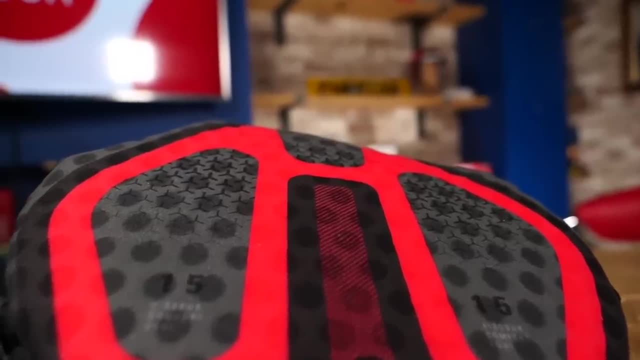 It might be a little bit bizarre, but trust me, you do get used to it. If you do happen to wear underwear underneath your cycling shorts, you will shave a lot and it will not be very comfortable or pleasant on the bike If you do see someone with underwear lines on the bike. 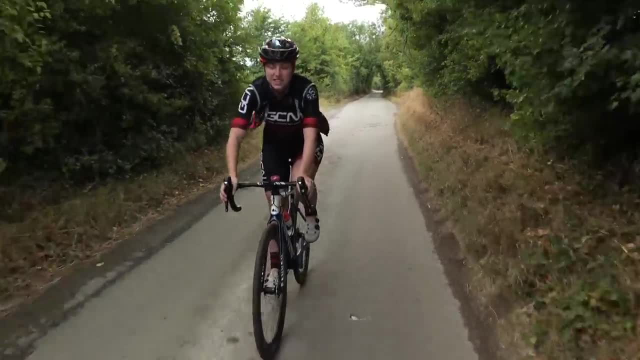 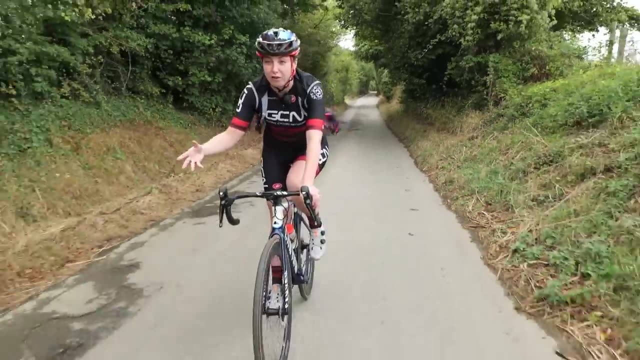 just give them a little nudge to tell them they don't need to wear underwear. take them off- Although I still haven't quite found a way to tell someone politely, take your underwear off. you don't need to wear underwear underneath your cycling shorts. 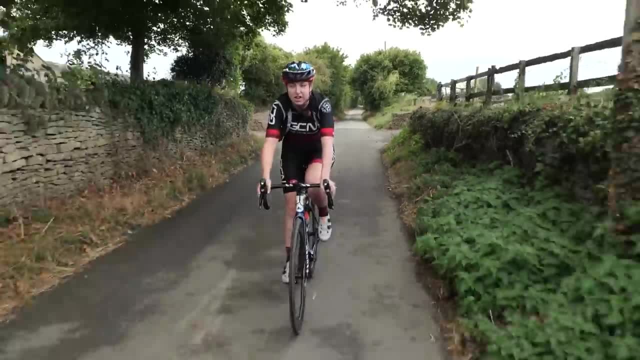 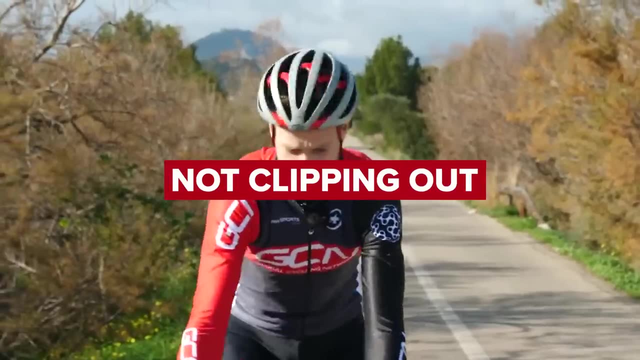 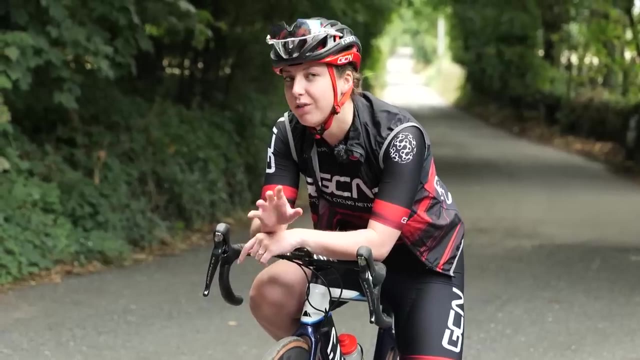 I know it does seem weird, but, as I said, our cyclists are a weird bunch. Just go commando, Be free. Now this next one has to be the worst feeling in the world when you can feel yourself falling in slow motion. At some point in your cycling lives you'll fall down the hole of clipless. 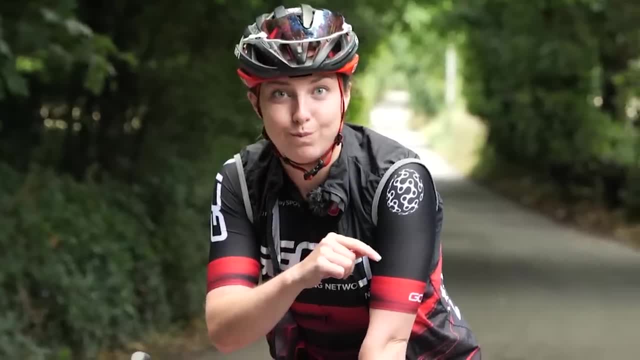 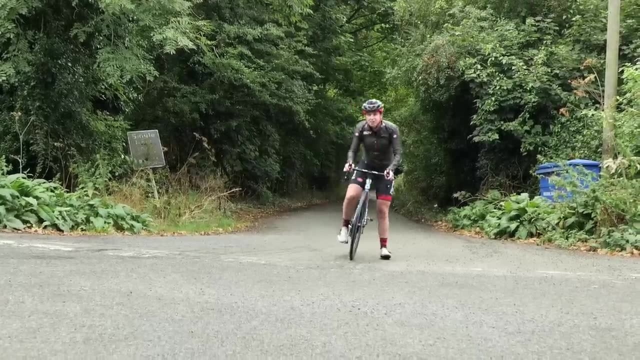 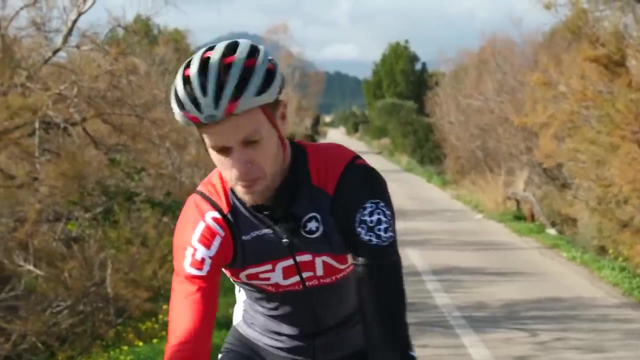 pedals. Now they're great when you remember to clip out. You're just riding along enjoying your ride and you come to a junction. Then you completely forget that you're pretty much attached to your bike. You try and unclip your foot from the pedal, it just won't budge. The next thing: 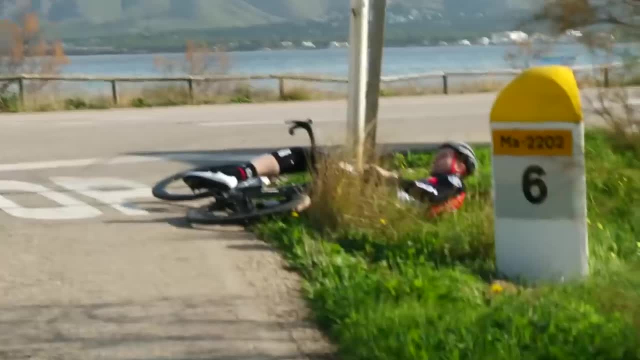 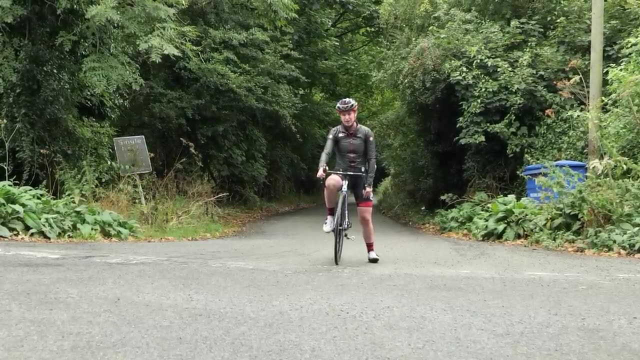 you're falling over in slow motion. You can feel it happen. The panic, the fear it rushes through your body, but there's nothing you can do. It's too late now. Then you're laying on the floor and everybody's looking at you and it's quite embarrassing that you have to get up. 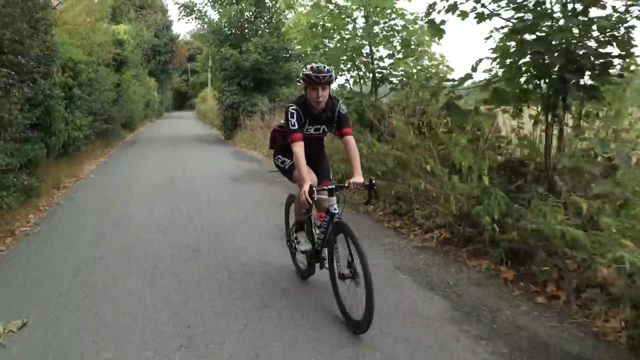 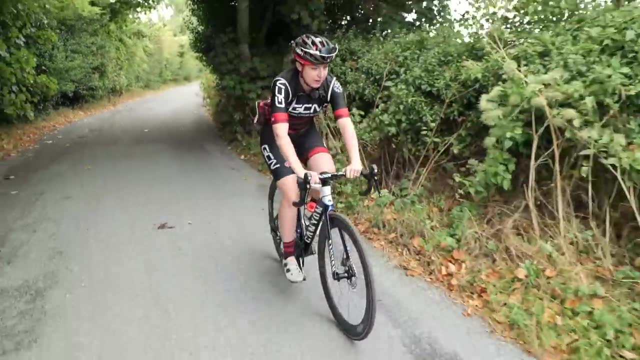 I missed the bean bag. Now, if this has happened to you, do not worry, We have literally all been there. Anybody who has tried clipless pedals has fallen over whilst trying to figure them out. A little piece of advice before you head out on the open. 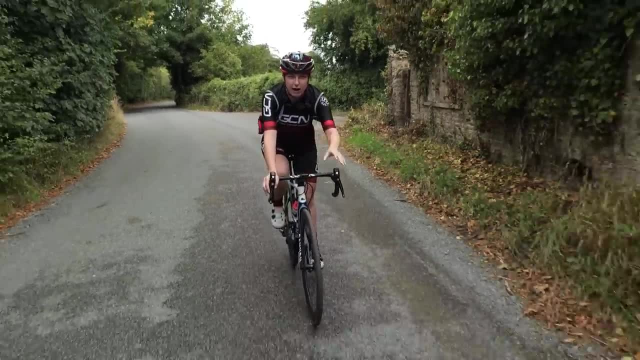 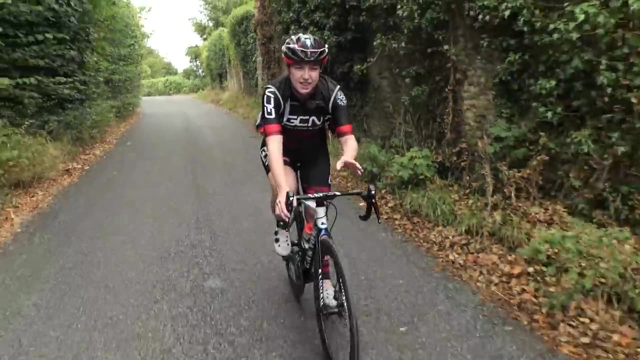 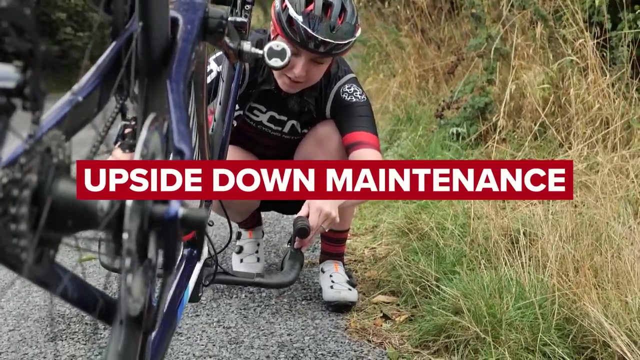 roads using your new clipless pedals. have a little whirl around in the garden, learn how to unclip quickly, learn how the maneuver works. It also helps to do it on grass. It gives you a bit of a softer landing. speaking from experience Now, when you begin cycling, a bike's a bike. 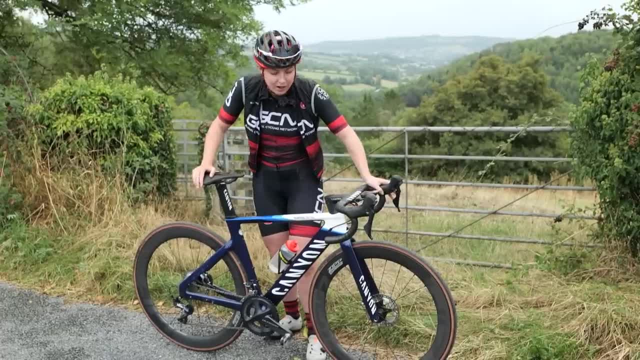 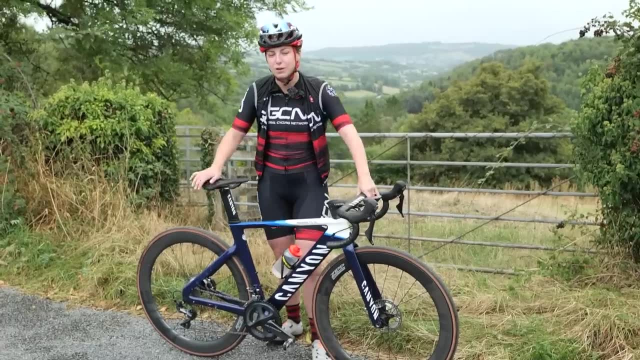 but very soon, as you grow to love our sport of cycling more and more, this bike will become your pride and joy. It's only a matter of time before it does happen. One of the biggest mistakes we see in beginners is when they do this To do any sort of mechanical. 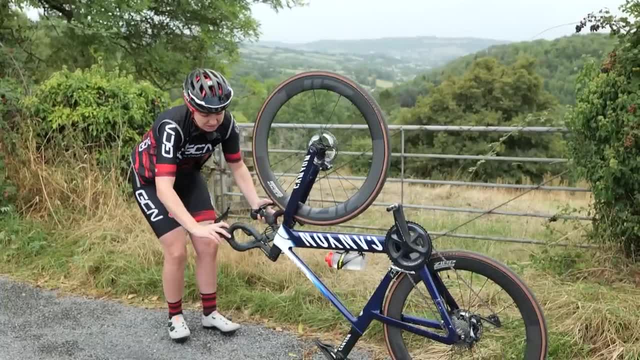 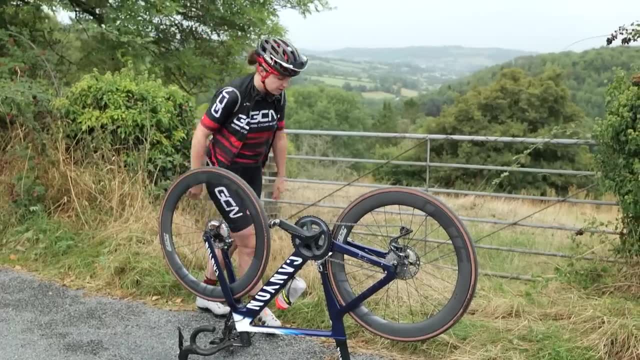 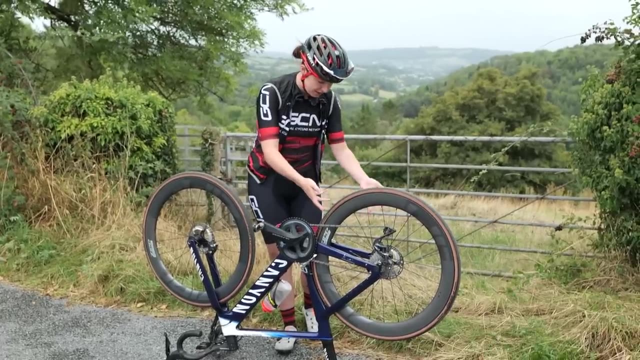 thing to their bike. they'll flip their bike upside down and rest the bike on the saddle and the handlebars. No, no, no. To me it doesn't really make any sense. Everything's upside down, which confuses things. I'll be honest, I can't even put a rear wheel in when the bike is upside. 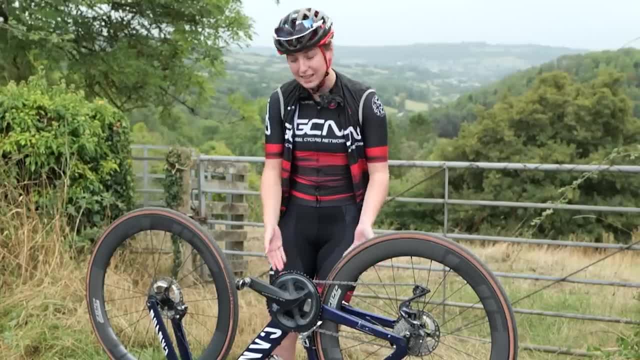 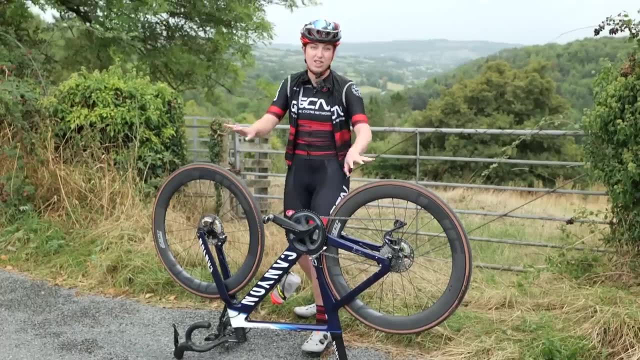 down Like this. Not only that, your saddle and your handlebars are touching the ground, They could scratch, and plus a gust of wind could come and it could just knock the bike over. then you'll have scratches all over your bike. You do not need to do this If you do need to do any mechanical. 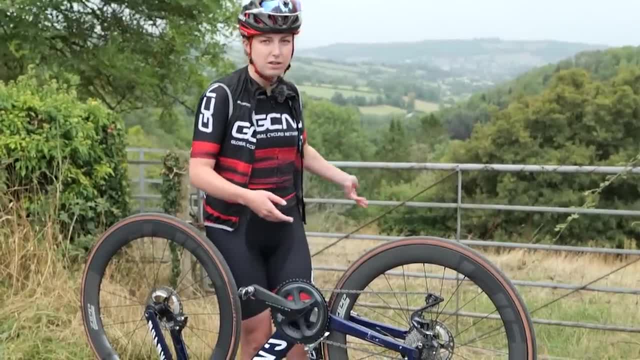 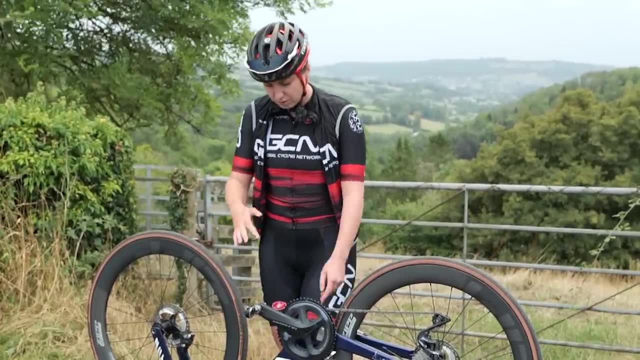 assistance to your bike. you could lean it up against a fence or a wall that doesn't scratch it, You could get a friend to hold it, or you could even just hold it up yourself and do some tweaking. Just don't do this. I'm so confused. 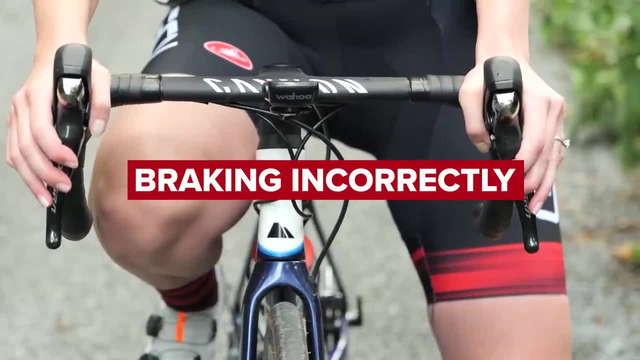 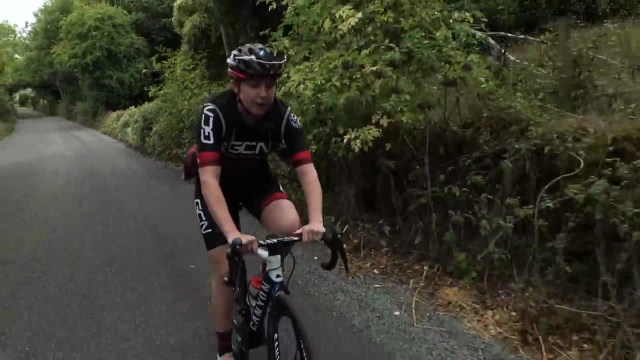 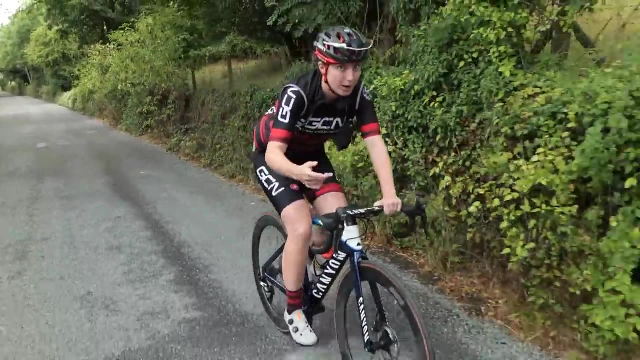 Now, once you get the hang of this one, you won't even need to think twice. but in a lot of beginner riders we see A them not knowing the difference between their front and their back brake B just using one. 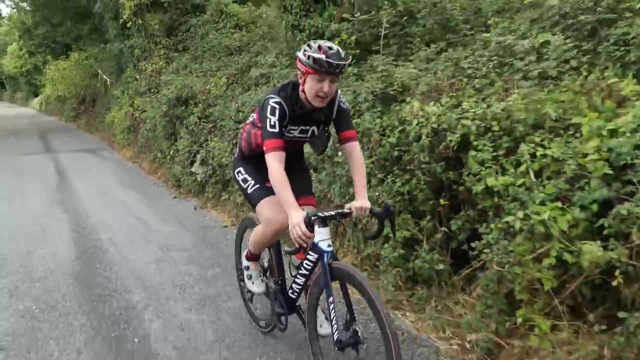 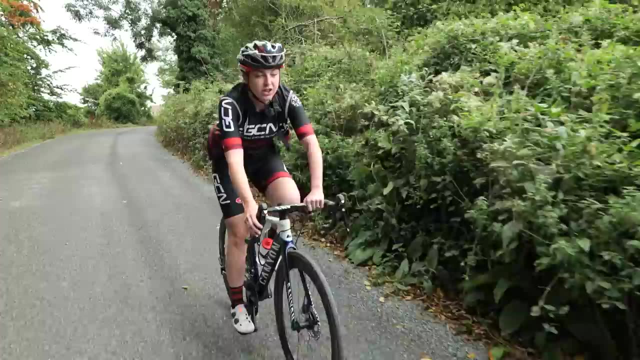 brake at a time and C not knowing how much brake they need to use to come to a stop. It's especially important to know the difference between your front and back brake. You can do this by standing up and just spinning the wheel and then just pulling one of your brakes. You can figure out. 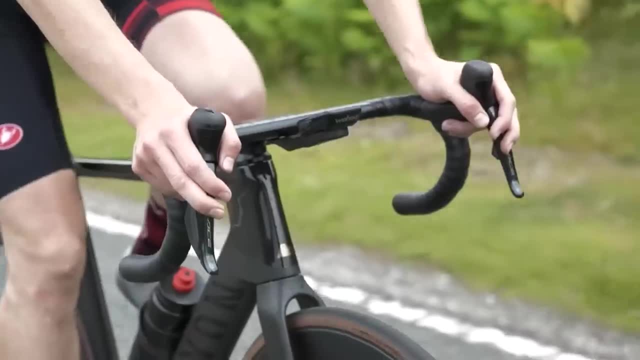 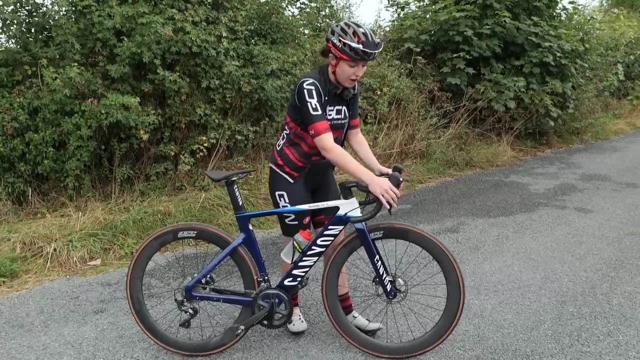 what is your front and what is your back? It's different on every bike depending on where you are in the world. Basically, if you pull your front brake- and just your front brake- very hard, this is essentially what's going to happen: You're going to fly over the top of your bike. 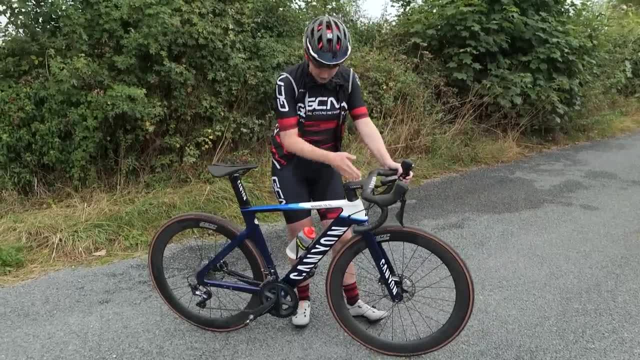 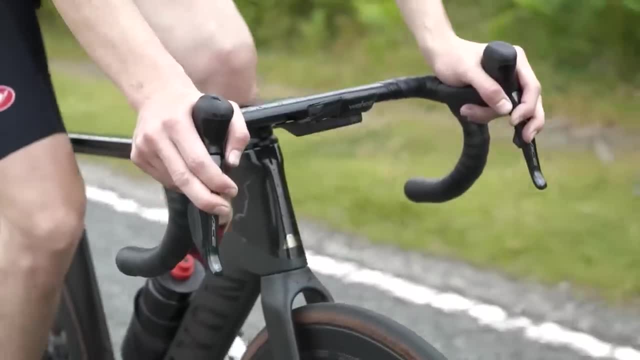 and that's not going to be very nice. On the other hand, if you just pull your back brake very hard, you're going to be scaredzilla. That's not good either. Also, how much pressure to put on the brakes to come to a stop. This one, you get used to it. the 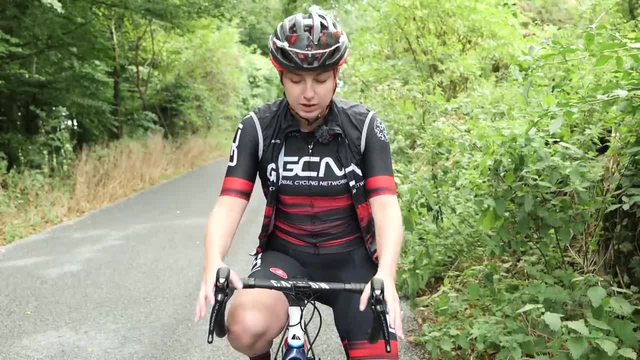 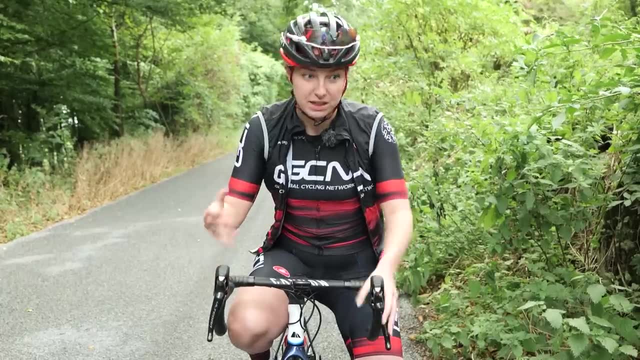 more and more you ride and you literally get a feel for it. Most of the time it's more of a feathering technique. to come to a stop, You don't need to take a big handful of brake and pull them to stop, because you will stop very abruptly. It's more of a feathering technique and I 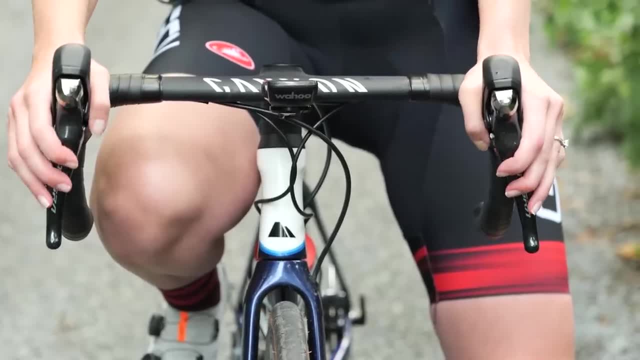 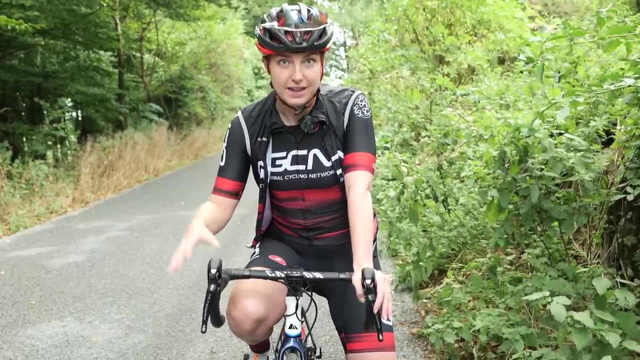 tend to use both the brakes, just feather them at the same time. If you are riding a new bike or you're not very used to the brakes on the bike, I recommend just having a ride around on the flat, Just getting used to them, see how sensitive they are, before you go zooming down. 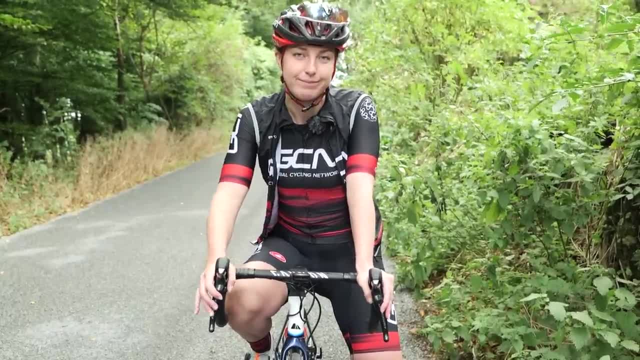 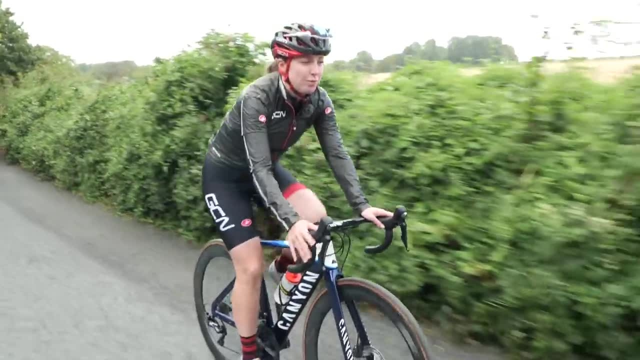 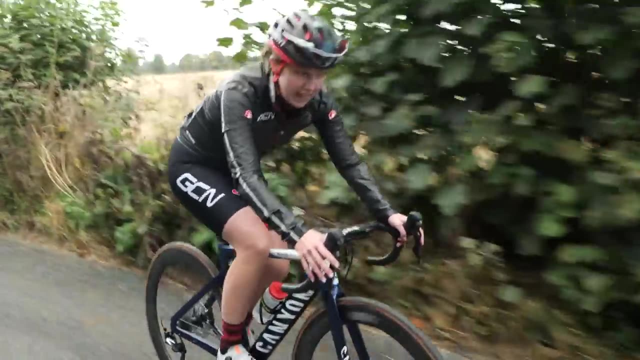 a massive descent, because that's a recipe for disaster as well. Gears are your friends When you learn how to use them. they make cycling so much easier. but you do see a lot of beginner riders riding around in the wrong gear. They'll either be riding in a massive gear like this one, grinding their way. 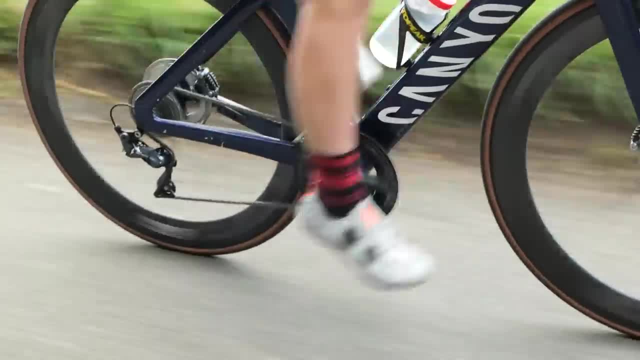 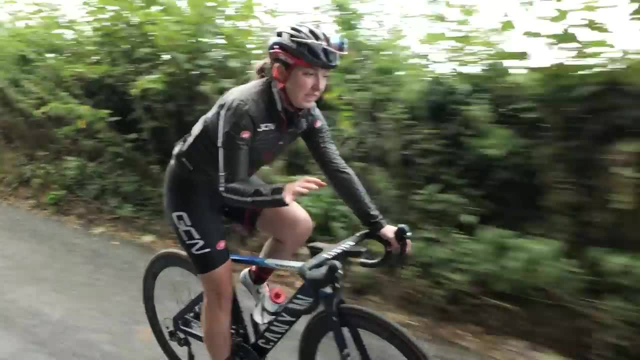 through the lanes or they'll be in the easiest gear, spinning their legs really fast like a cat on a wheel. The sooner you learn how to use them properly, the easier the riding will be. I'll be honest, I had no idea how gears worked when I first started cycling. 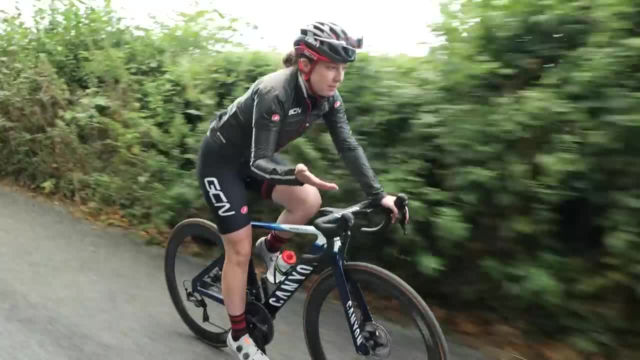 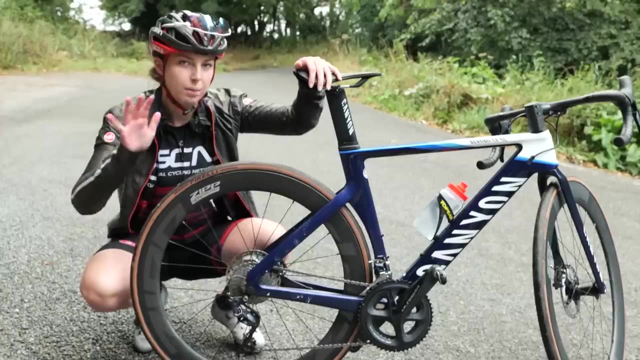 didn't know how to change gear and I had no idea what gear I needed to be in when I was going up a hill on the flat or anything. Let me try and explain To keep it nice and simple. if you're going up a very steep climb, you need to be in your easiest. 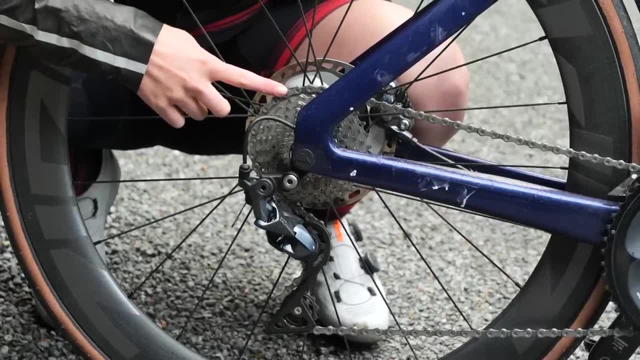 gear. This is pretty much having your chain in the middle of the bike. If you're going up a very steep climb, you need to be in your easiest gear and this is pretty much having your chain in the middle of the bike. This is pretty much having your chain in the middle of the bike. If you're 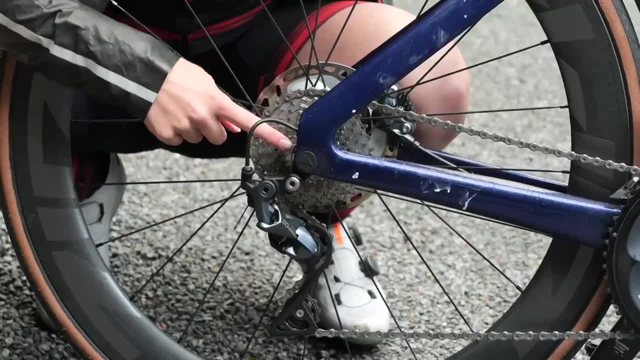 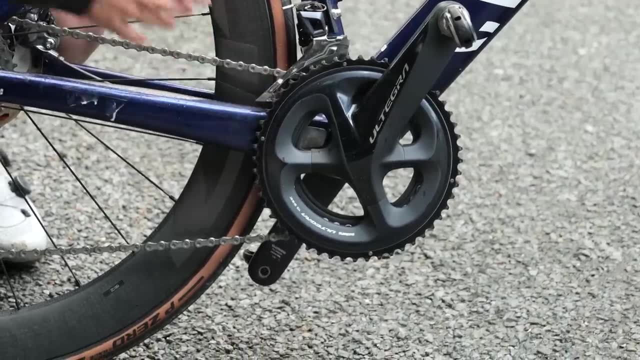 going on a flat road or a downhill road. you need to be in the smaller cogs down here, going uphill in the little ring, going downhill on the flat big ring. Simple, It's not actually that simple. There's a lot more to it. You can then go into. 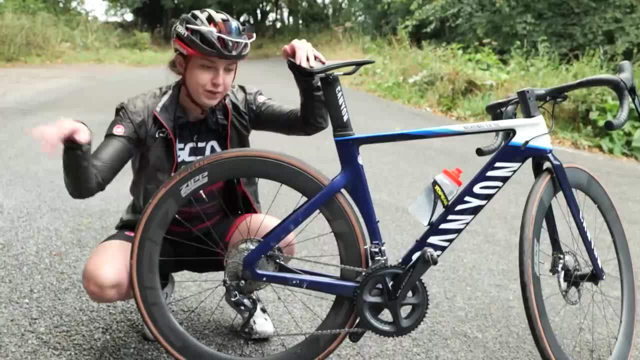 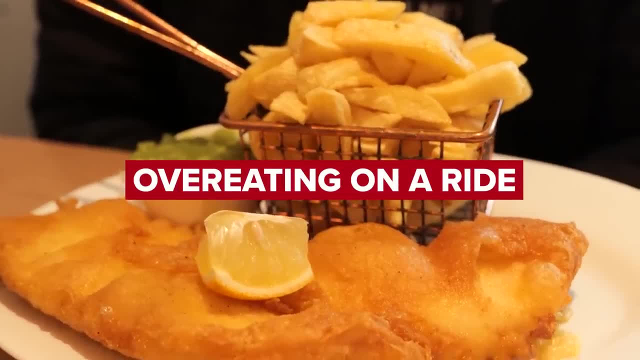 RPM, leg speed- all that, which is a whole another kettle of fish. If you did want to learn more about that, we've got other videos on the channel. Now don't get me wrong: Stopping at a cafe on a ride is always. 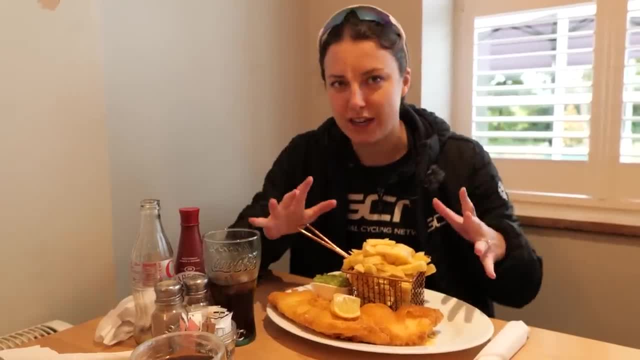 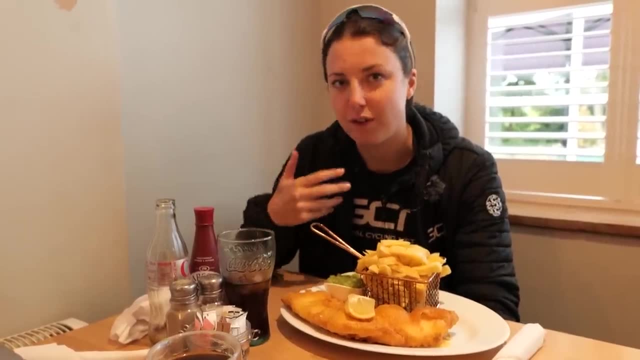 a good idea, but one mistake you can make at the cafe is ordering too much food, because eating a massive meal like this, for example, when you get back on the bike, you're going to be very full, very sluggish and very sleepy and you're just not going to want to ride a bike. Try.